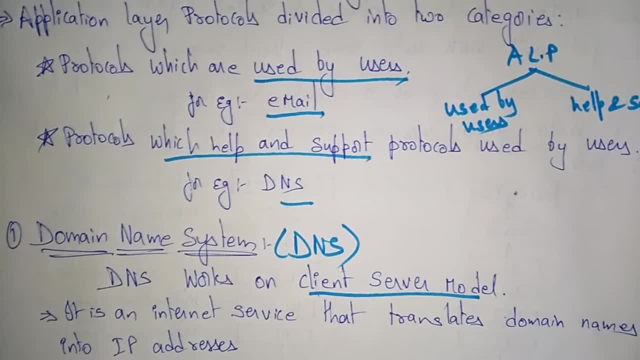 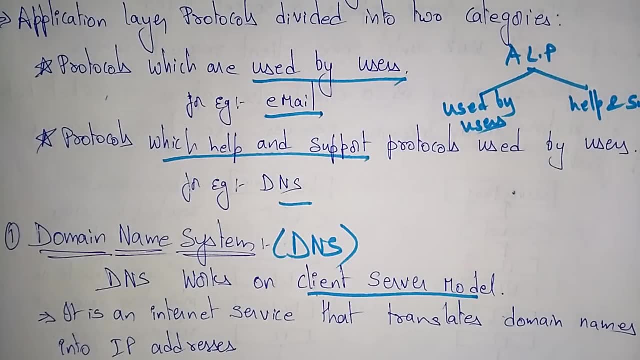 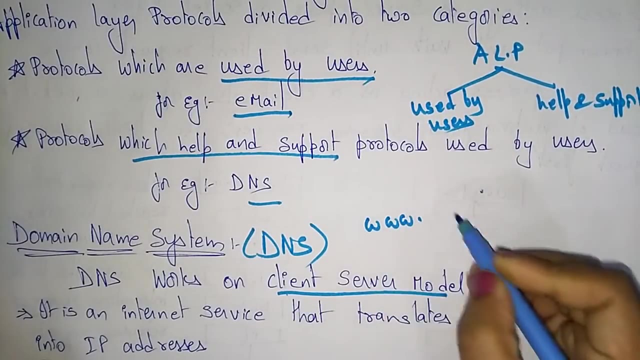 it is an internet service that going to translate domain names into ip address. so whatever we are giving that domain name is going to convert it into ip address. what is a domain name actually? so let's take a wwwlet's take gmailcom, so this completely, you call it as a domain name. 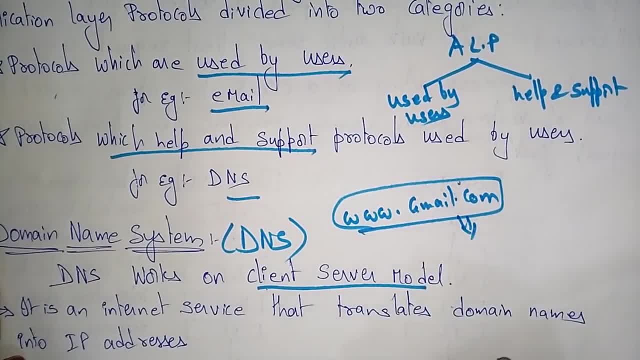 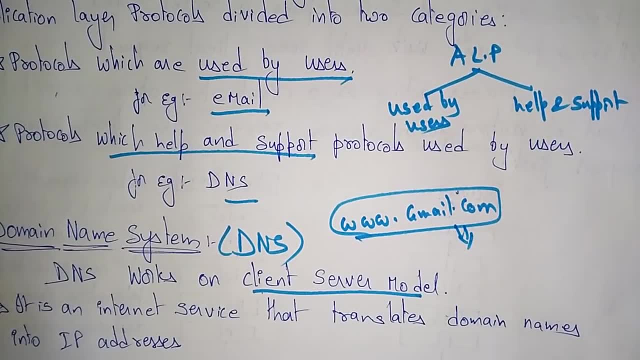 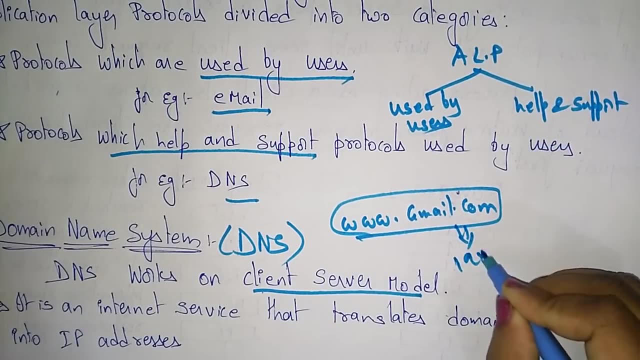 so this domain name is going to translate into ip address. then only the system can understand. the network layer can understand only the numbers in the binary format. so first this domain name is converted into decimal numbers like suppose 198, point something, something dot like, and again this will be converted into binary format like that. then the network layer can. 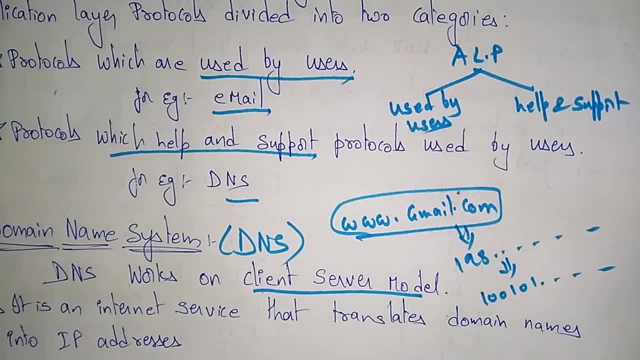 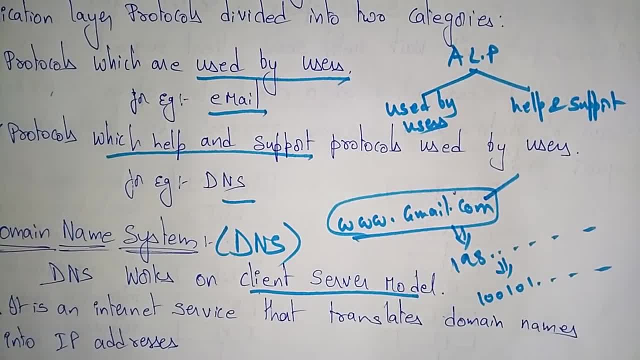 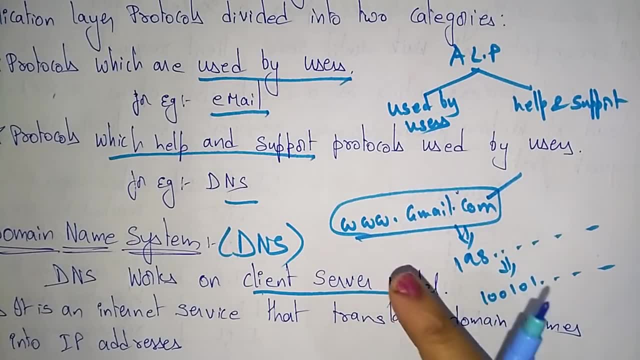 okay, service system that is uh present in the application layer that the user can interact, that is used by the user and uh this will uh this domain name system which helps and support the protocols used by the user. okay, so don't be confused. dnsn works as a client server model. 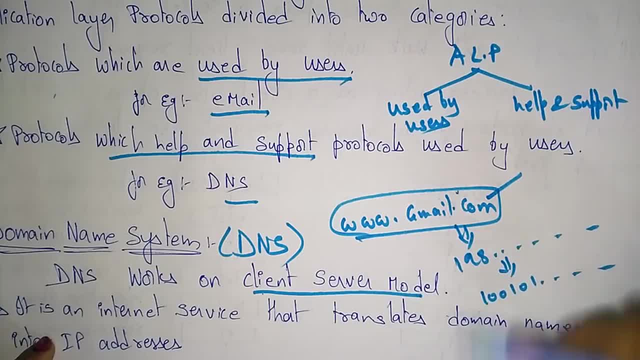 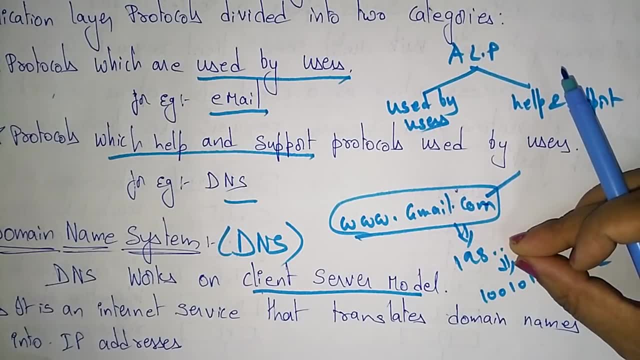 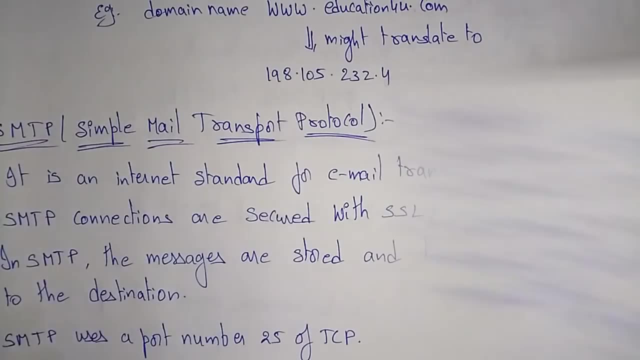 the first thing. and next, it is an internet service that translates the domain name into: so this is a domain name. this domain name is translated into ip address with the help of the domain name system. okay, so let's see here the example: a domain name: wwweducation4ucom. okay, this is our site. 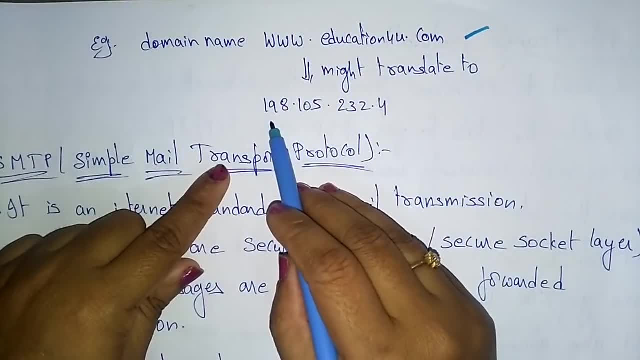 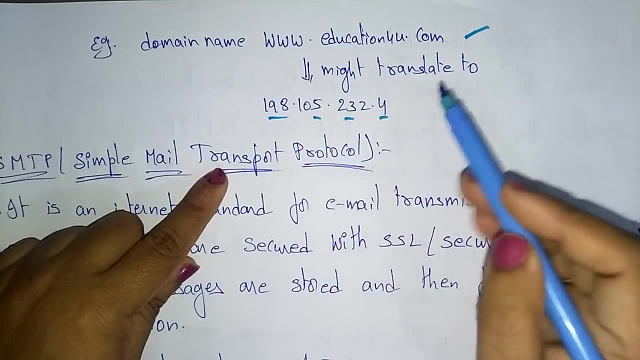 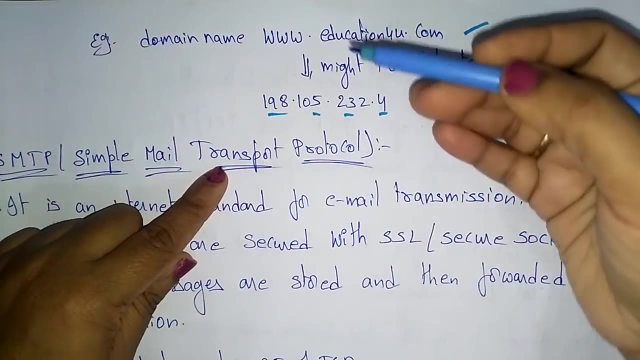 so this might be translated to one eight, one ninety eight point one zero five dot two. thirty two dot four. okay, each octant it specifies the address where exactly that location was that? so, with the help of the domain name system, uh, we can understand the domain name.